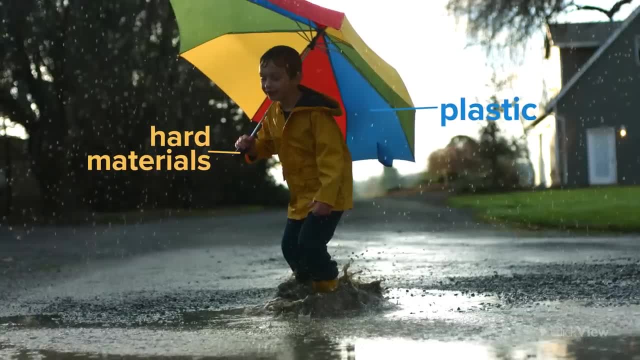 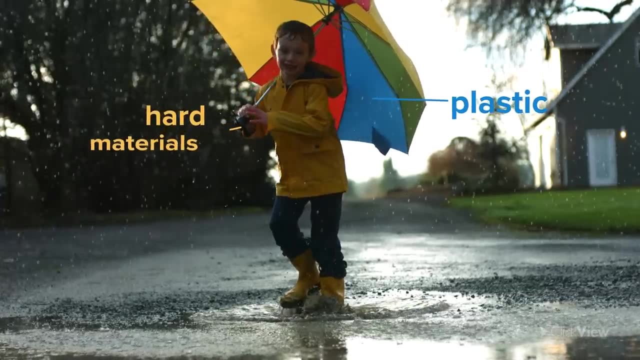 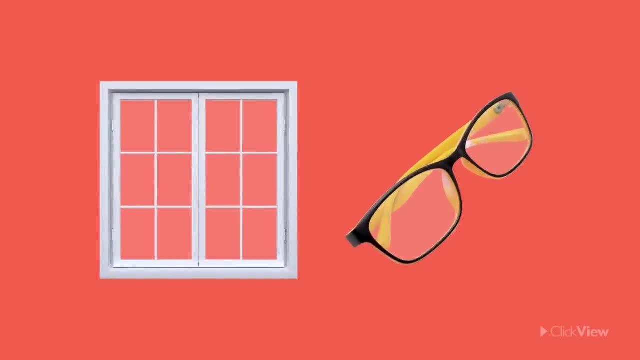 And the plastic was chosen because it is waterproof and light, which lets the rain drip off while allowing you to carry it easily. Why do you think we use glass for windows and reading glasses? You've probably already guessed it: because you can see through it. 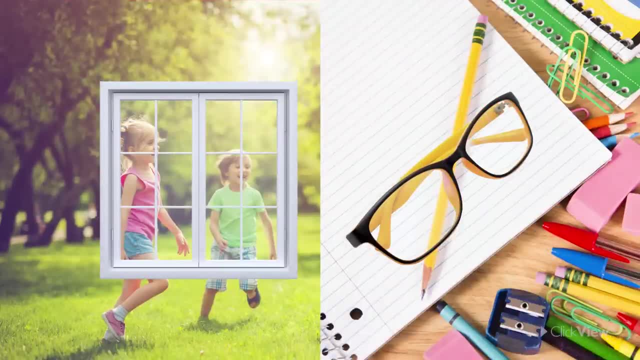 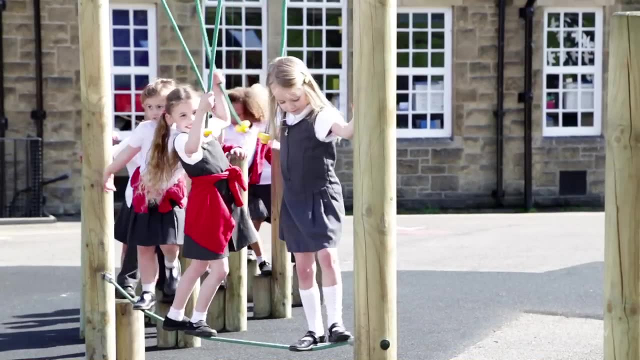 These objects wouldn't be much use if they were made of wood, would they? You may have noticed that the glass is made of wood and the glass is made of plastic. You may have noticed by now that our clothes are made out of special materials as well. 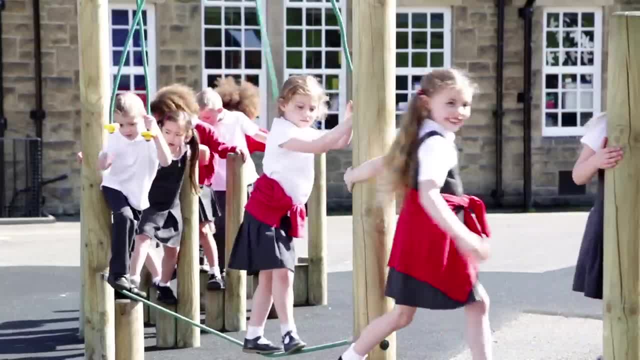 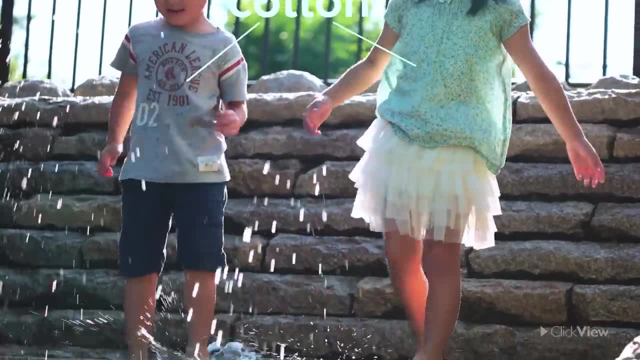 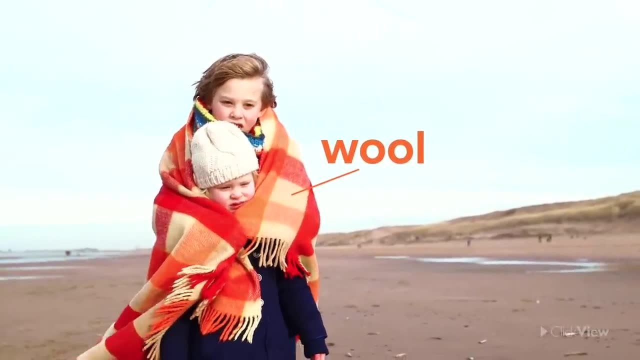 and these materials also have unique properties. Can you guess what materials your clothes are made of? They might be cotton, which is a fabric that helps you stay cool on a hot day, Or they might be made from wool, which is very good at keeping you warm on those cold winter days. 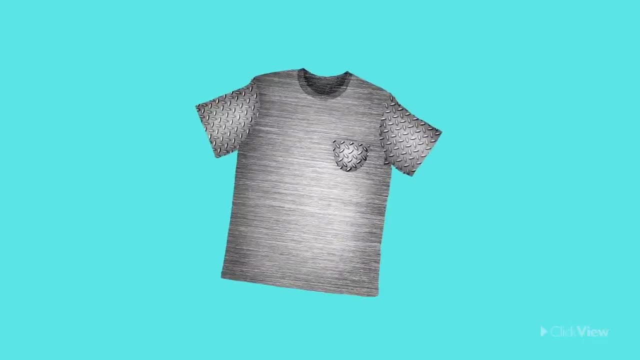 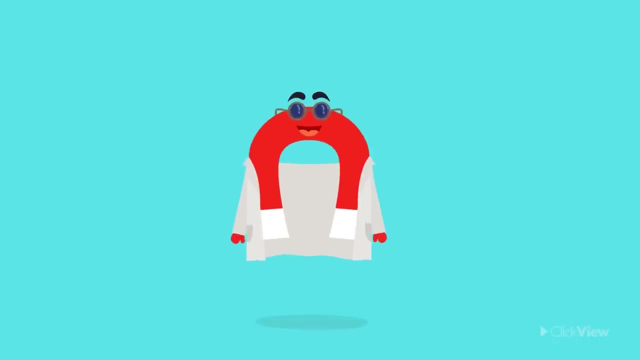 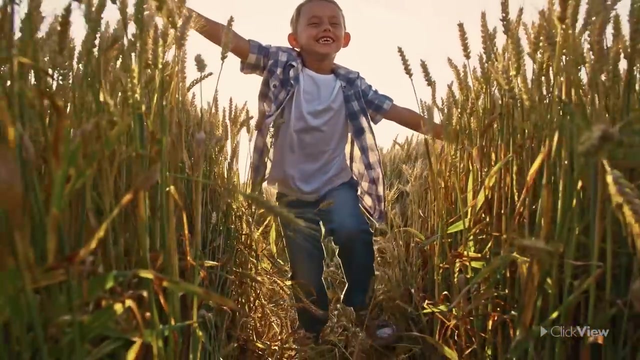 What do you think would happen if you wore a T-shirt made from metal? Well, that would just be silly, wouldn't it? You wouldn't even be able to move. Can you now see why we choose certain materials for our clothing? They let us move easily and stay comfortable, because they are flexible. 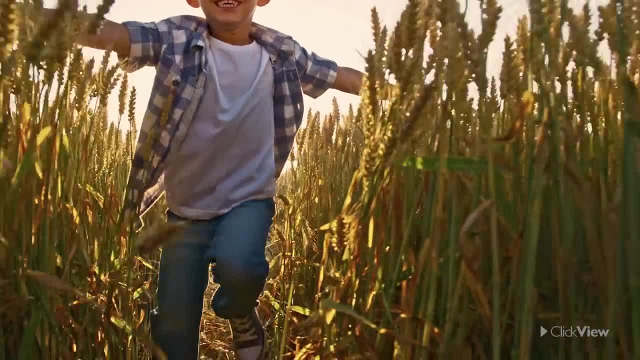 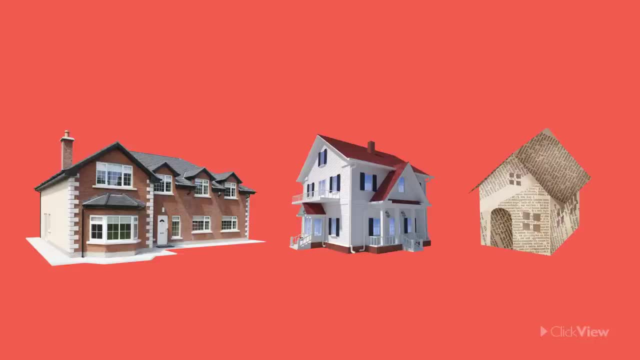 and help us keep warm or cool, depending on the weather. Now, which of these houses is different from the others? Of course, It's the house made out of flimsy paper that is different. Have you ever seen a house built from paper? 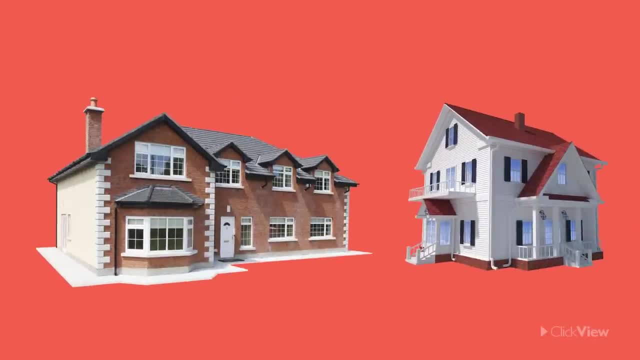 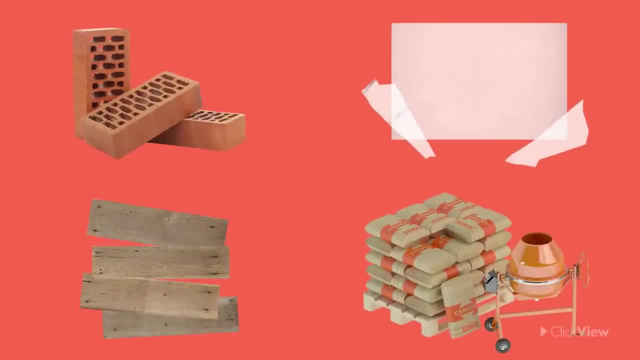 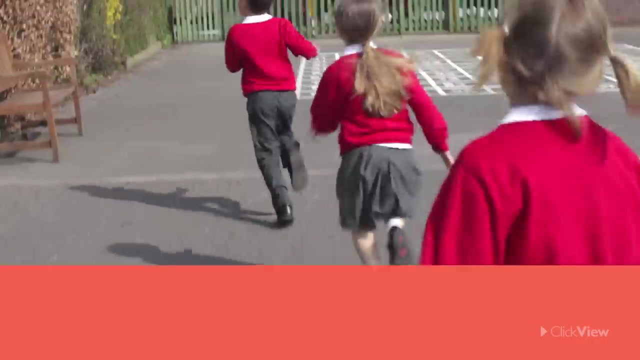 No way. When it comes to building houses, we need to use tough materials such as bricks, glass, wood and cement, so that they stay standing for a long time and don't blow over in the wind. Now that you know about materials and their awesome properties, 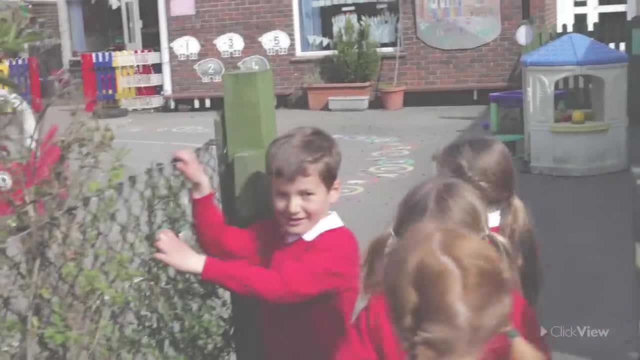 I wonder if you can spot something like this in some of them around your school.